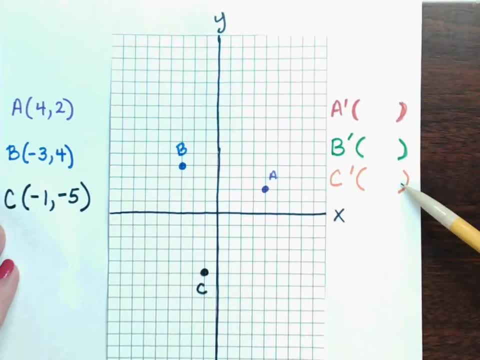 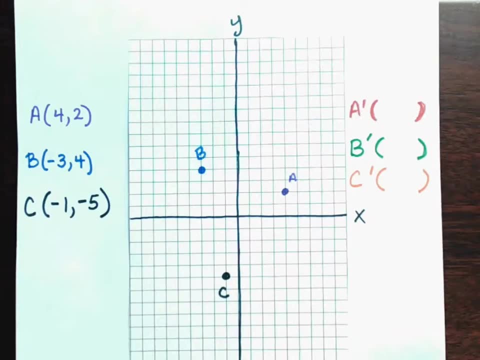 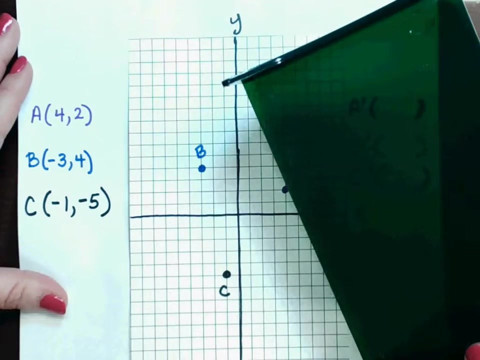 which will be the ending coordinates. I'm going to show you how to plot a point after I have reflected across the x-axis. Now I'm going to show you a couple of neat things that we can use to show reflections. This handy-dandy thing is called a mirror, not a mirror like we would look in to fix. 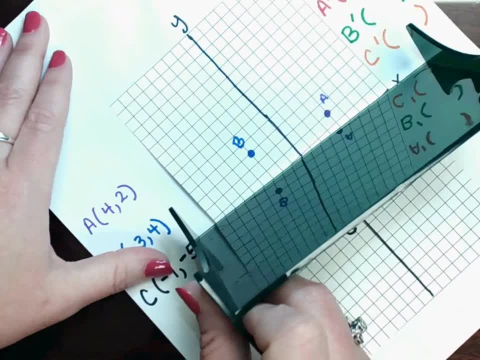 your hair or put on your makeup. but I'm going to lay it across the x-axis because that's what I want to do. I want to reflect each of these points across the x-axis. I'm going to lay it across the x-axis because that's what I want to do. 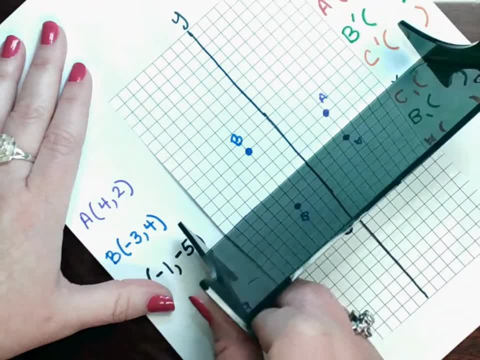 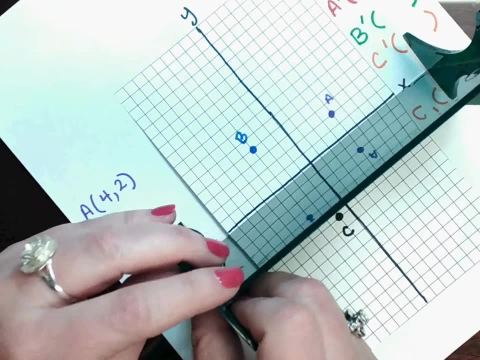 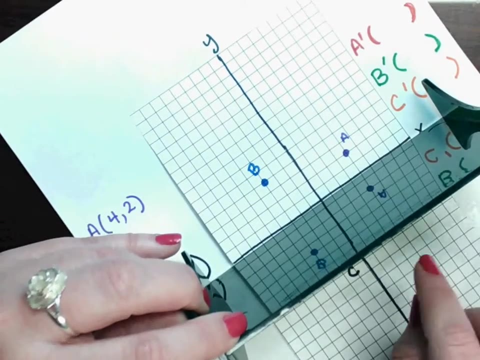 This handy-dandy thing is called a mirror, not a mirror like we would look in to fix your hair or put on your makeup. but I'm going to lay it across the x-axis, because that's what I want to do. If I lay it on the x-axis here, you can kind of see through the camera that the A' is. 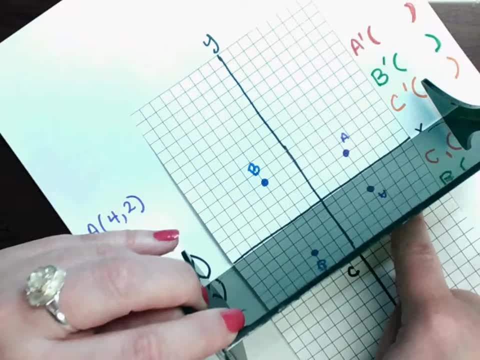 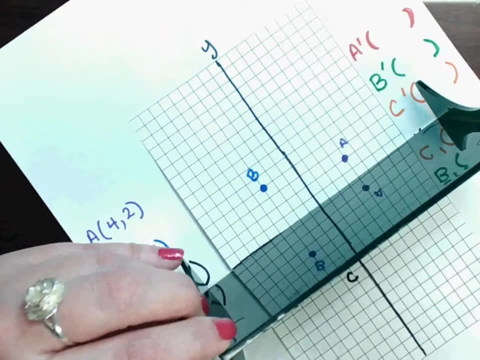 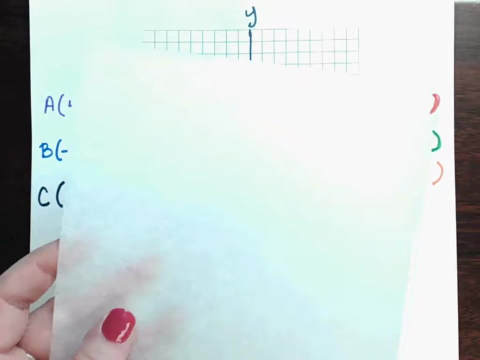 over here towards the back And you can kind of see that the B' is right back here also. but since you don't have these, this does you no good. But this is a neat little tool that you can use. There's also something called patty paper. 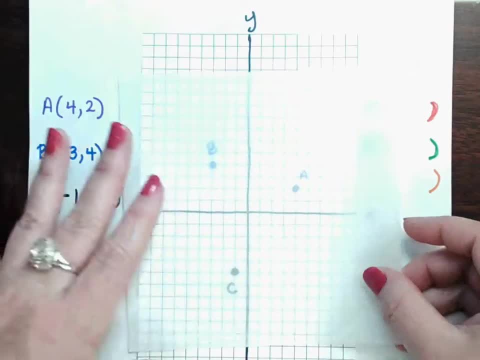 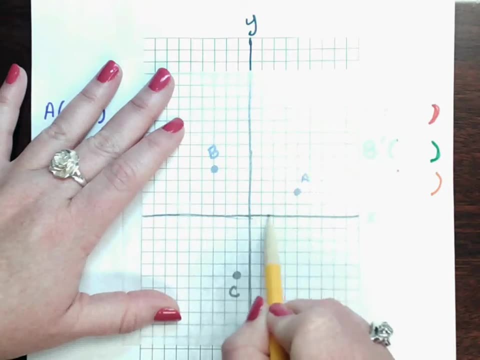 It's just like tracing paper, which I'm sure you've all seen. So how you would use this is you would lay it across the x-axis that you would want to flip across, Draw across the x-axis And then also trace the bottom. 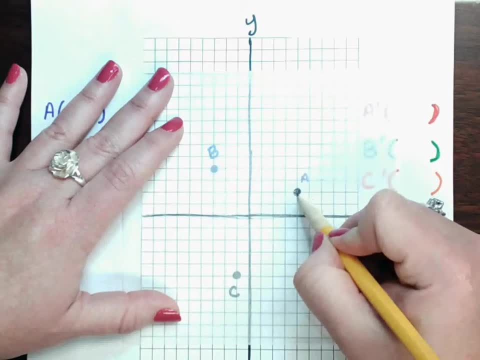 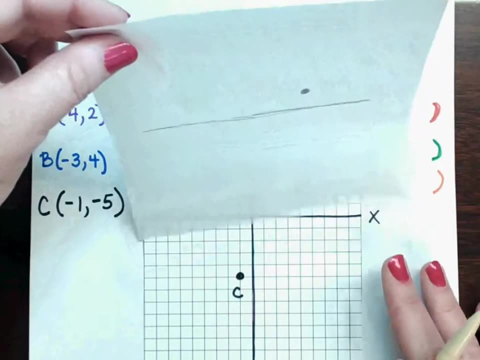 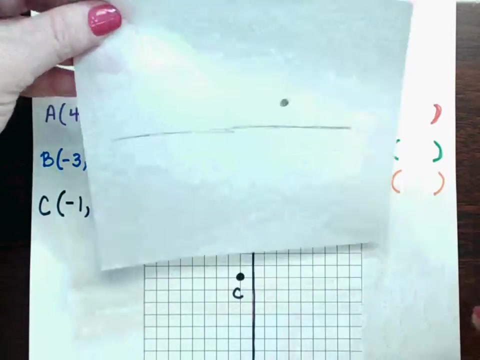 And then also trace the bottom And exactly is the point that you want to flip. So in this case we want to reflect the A point. Since a reflection is a flip, you would literally flip the paper. so see here how he paper has the axis and the point that I want to flip. 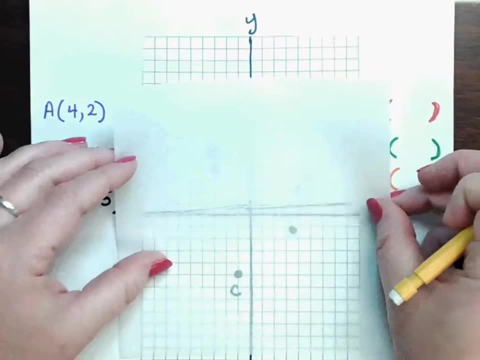 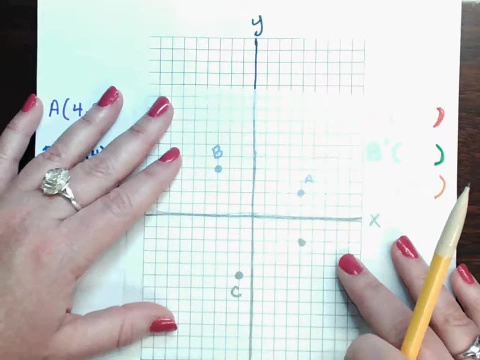 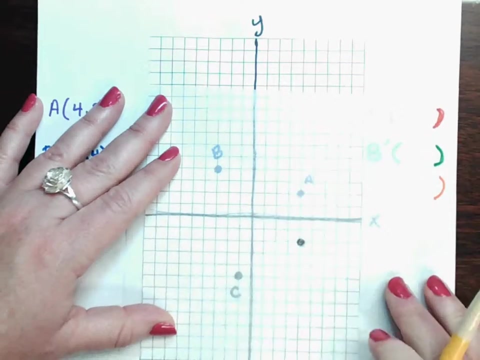 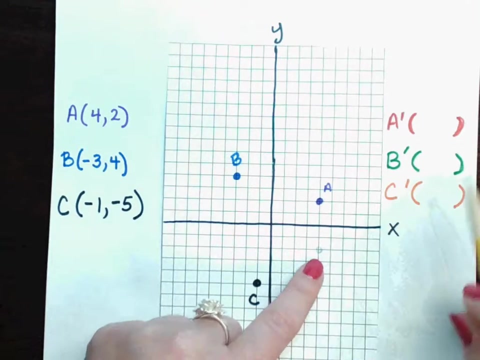 So you would flip it, Lay the axes on the axis, And then your point would actually Wait. How be? where your reflection would be so in this case, and you can see right here where the pencil mark made the point. now, if you notice anything, I'm going to go. 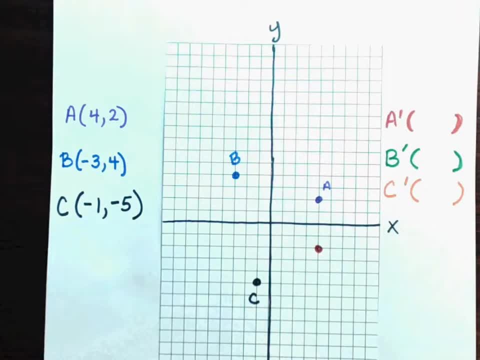 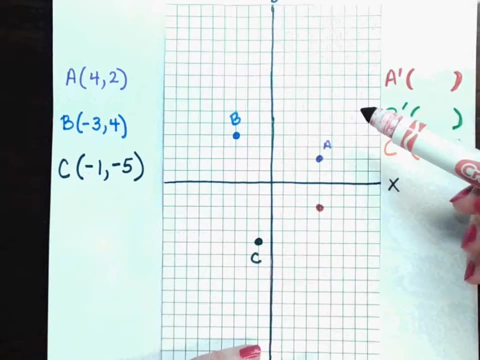 ahead and put this point here, and since most of you don't have patty paper, you won't be able to use this either. so let's figure out a way that we can easily reflect without having to use a mirror or patty paper. let's notice how. 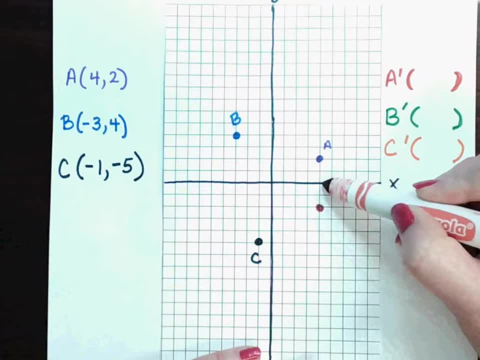 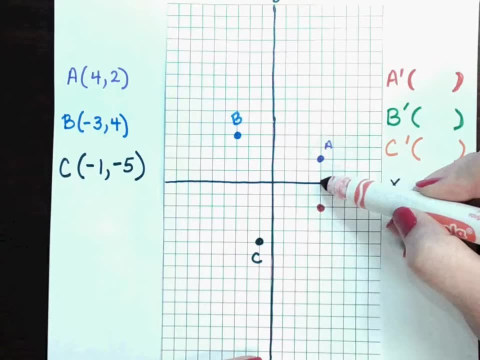 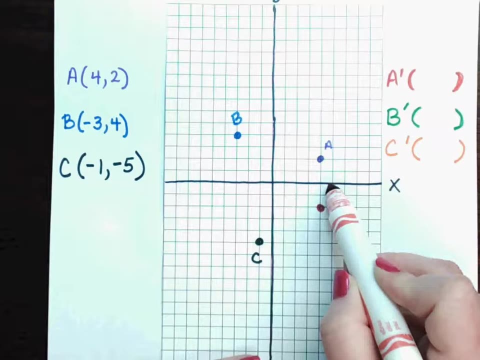 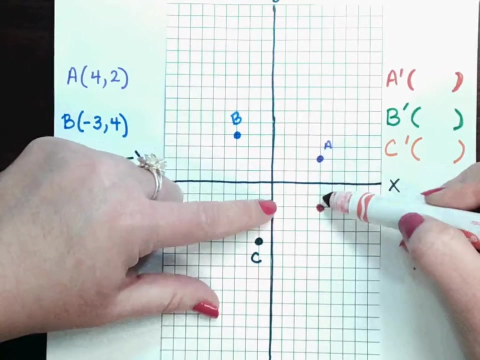 many. the reflection is away from the X-axis, so the reflection is one, two away from the x-axis, just like the original is one, two away from the x-axis. it's still the same amount across and it's still the same amount down, But in this case the point is shifted down instead of up. 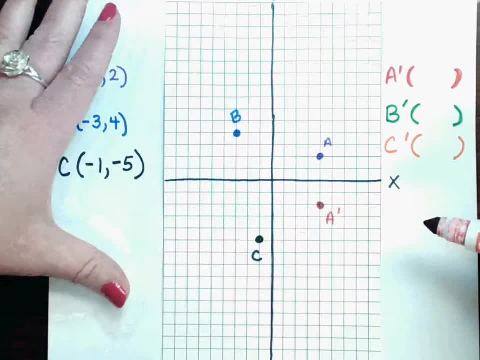 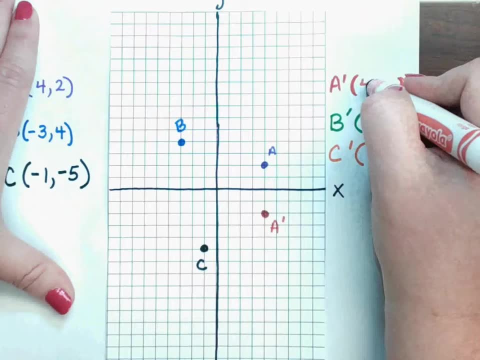 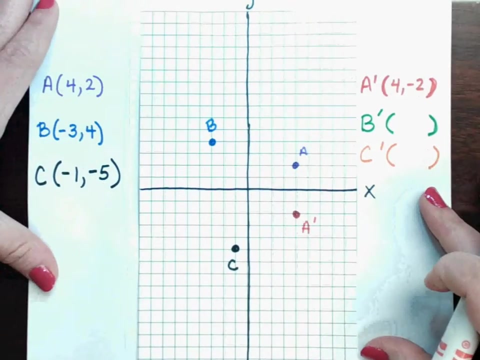 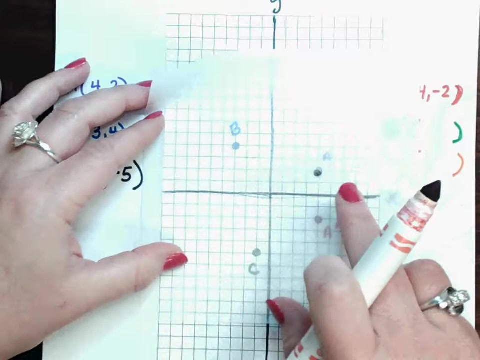 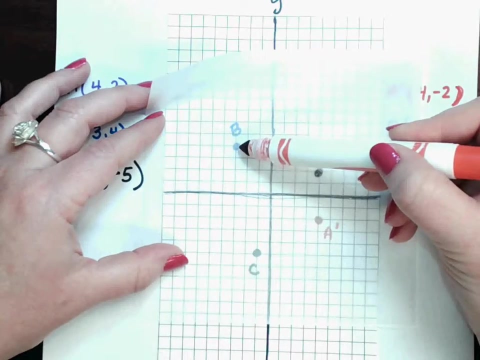 So I'm going to label this A' And my new coordinates would be 4, negative 2.. Alright, so let's look at B. Okay, keeping in mind that I could do this, if I were to trace B right here and then flip it, it should end up down here. 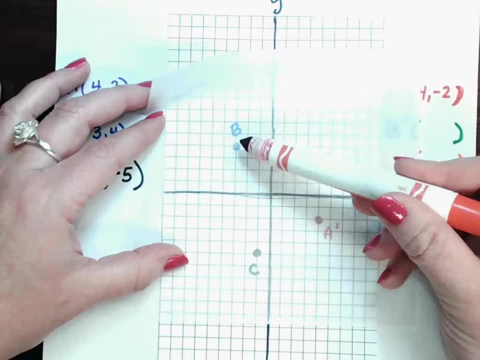 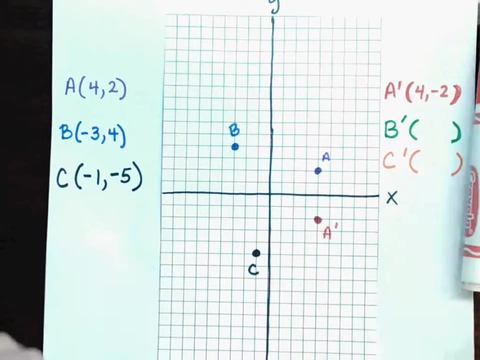 The same distance away from the axis as it was up here. So what I'm going to do is I'm going to count how far away B is from the axis here And then count, And then count that many away from it and put it down here. 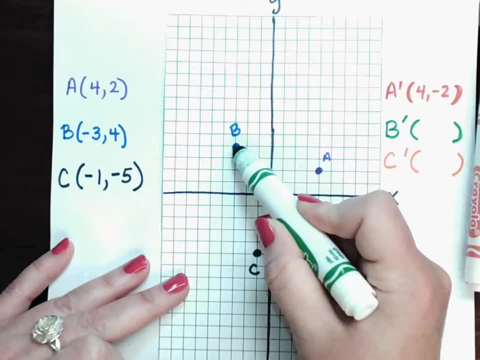 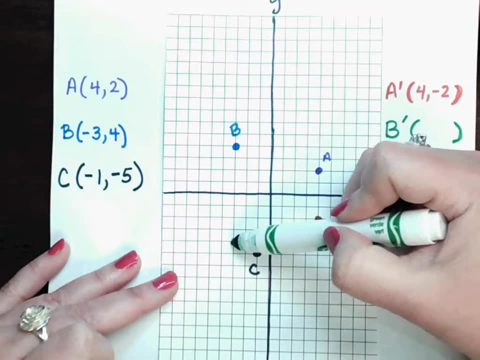 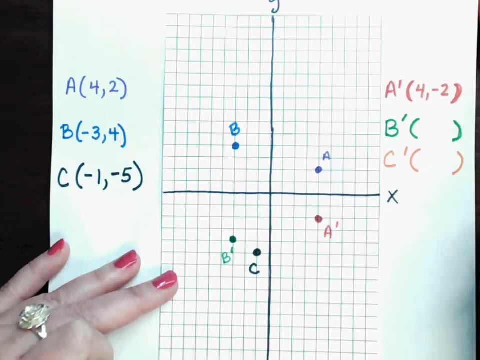 So it's 1, 2, 3, 4, up, So a reflection would be: 4 down, 1, 2, 3, 4.. So B' would be right here. So I'm going to go ahead and make that negative 3,, negative 4.. 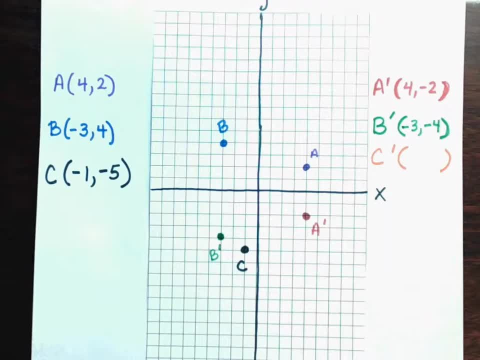 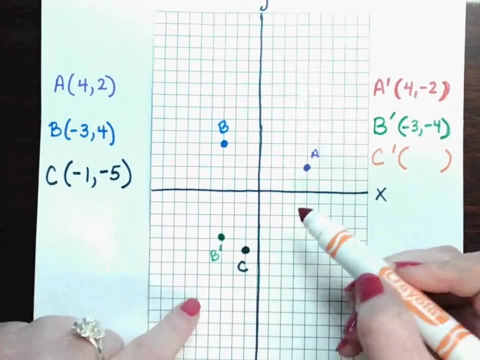 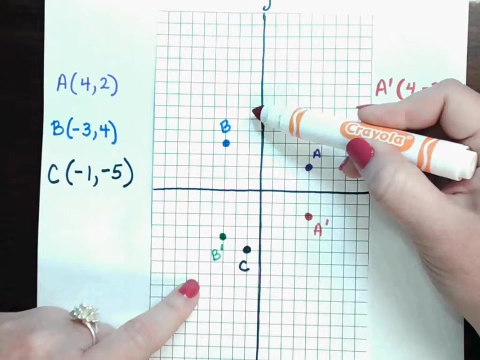 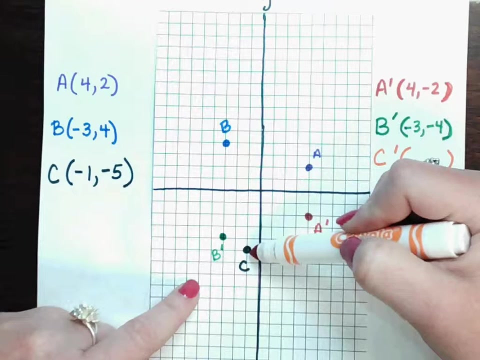 Okay, C is the same, except it starts out below. So when you would flip it it would actually end up here, above the x-axis. So if it's 5 below the x-axis, the flip is going to be 5 above the x-axis. 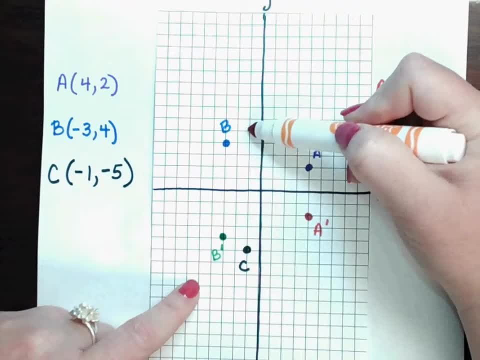 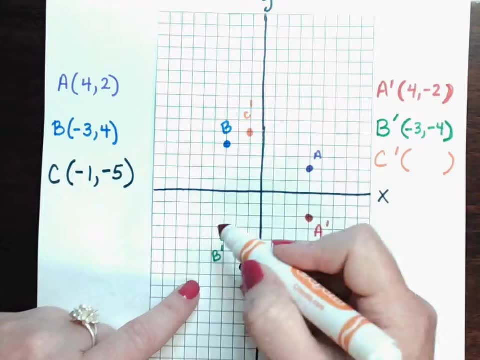 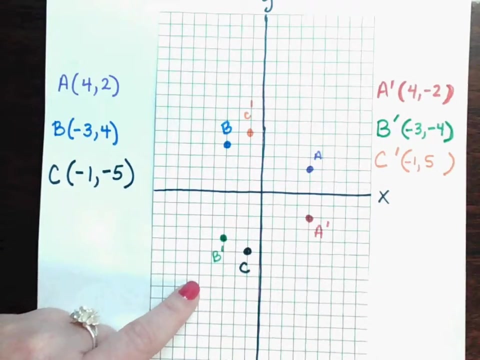 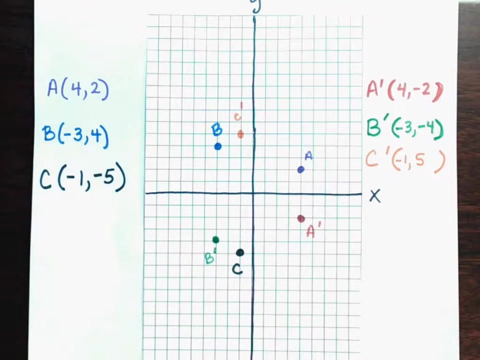 Okay, So 1,, 2,, 3,, 4,, 5.. So C' is going to be right there, So I'm going to go ahead and put my coordinates as negative 1,, positive 5.. Okay, Okay, so that was pretty easy because we just had single points here. 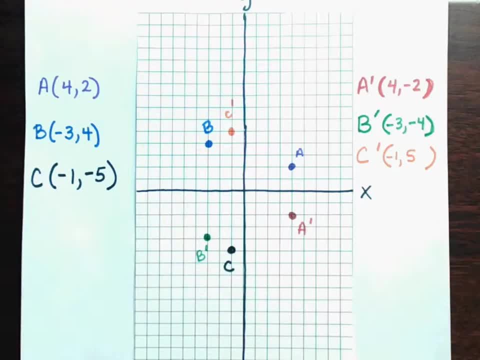 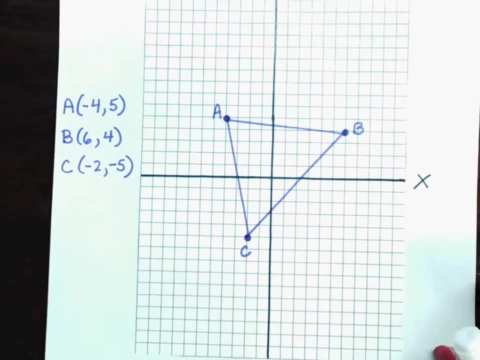 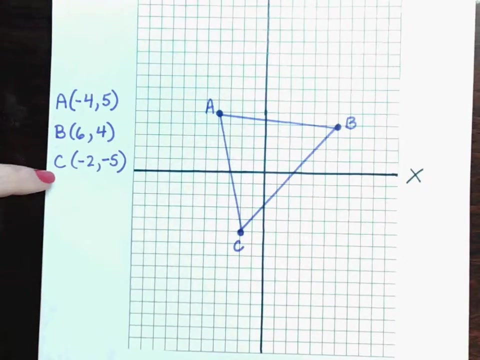 What if we wanted to reflect an entire figure? So let's look at this. We have an entire triangle that we want to flip. So we're given the coordinates for A, B and C. You're still going to do the same exact thing. 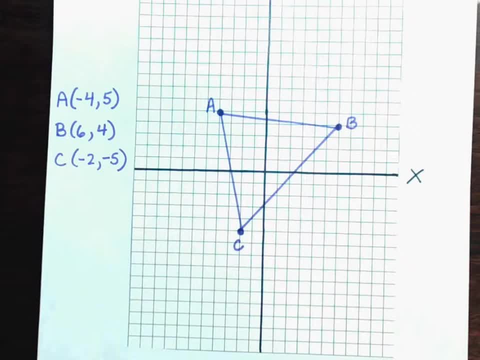 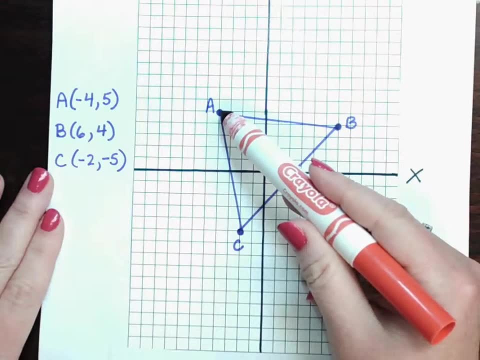 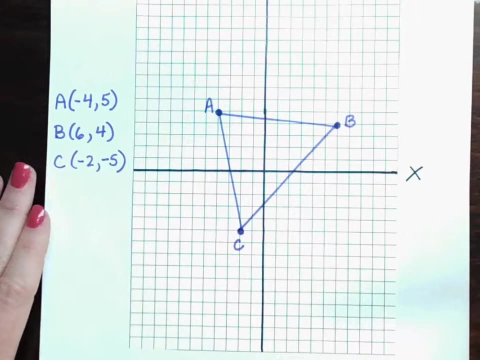 that you did for each individual point. So you're going to figure out how far away each point is from the x-axis. Okay, So we're going to go ahead and put the x-axis and then count that much further away from the x-axis on the other side and put the prime point. 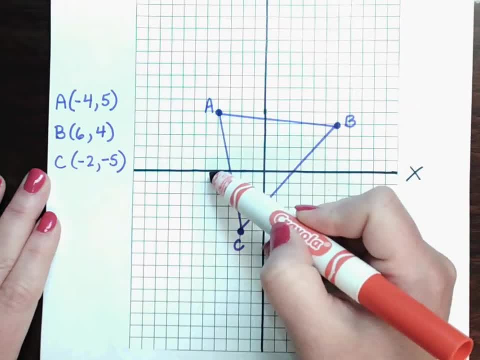 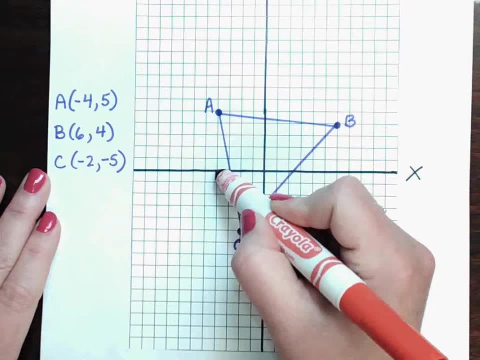 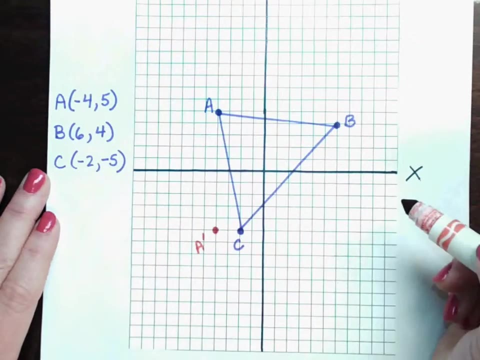 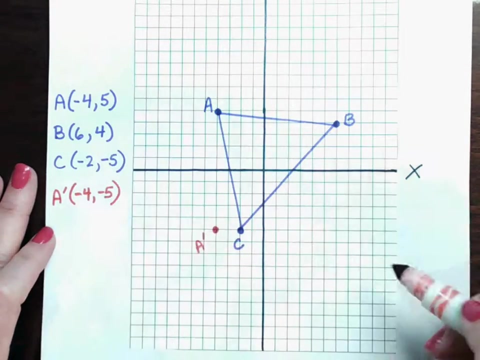 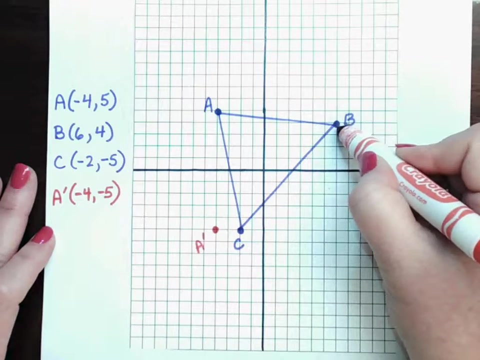 So in this case A is negative, 4 up, 5.. So the A prime would be negative, 4 down, 5.. So this is A prime, B is 6, positive 4, so if I reflected that would be 6, negative 4.. 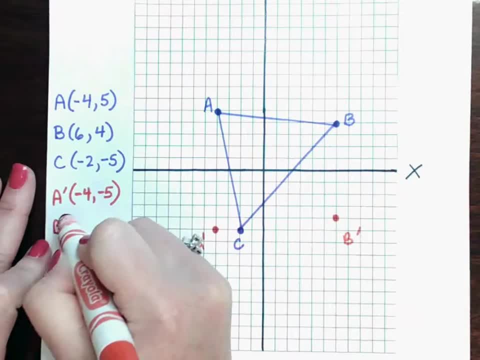 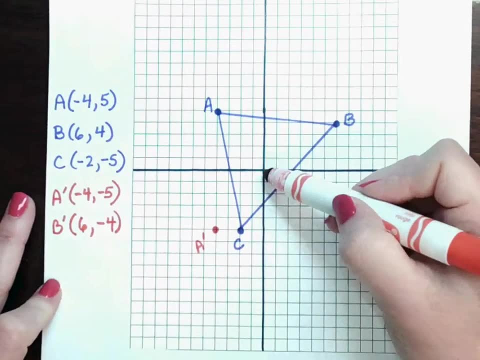 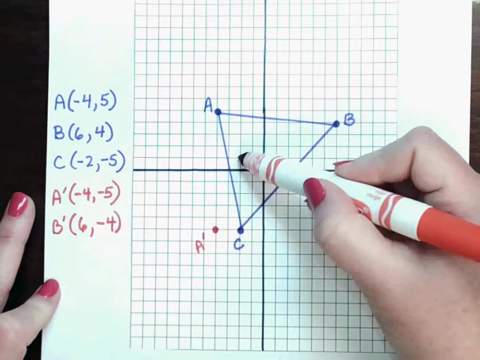 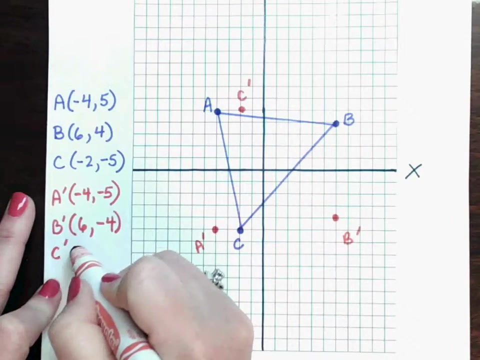 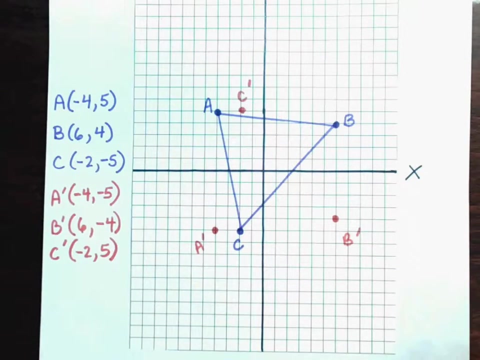 So that's your B prime. C is negative 2.. Negative 5, so this is going to be negative 2, positive 5.. And then you'll have to forgive me because I don't have a ruler. you're going to connect.